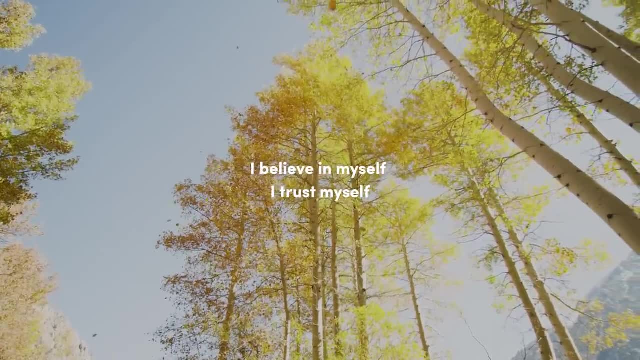 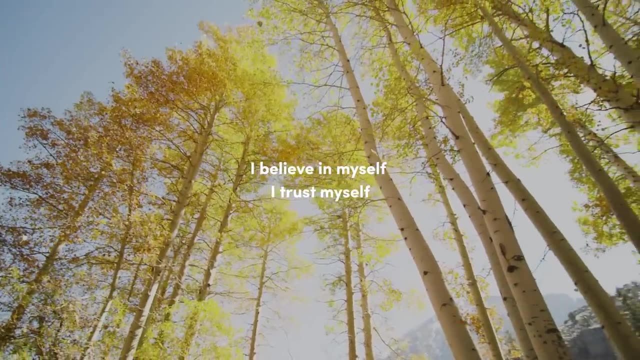 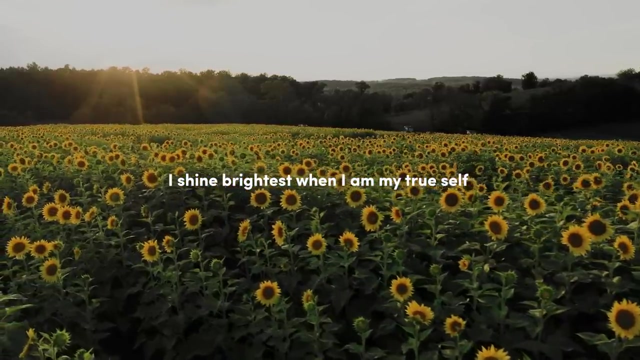 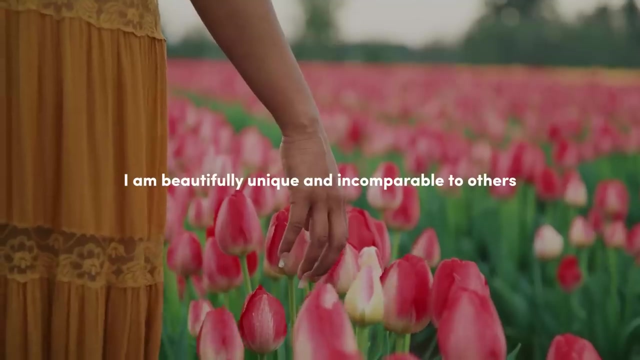 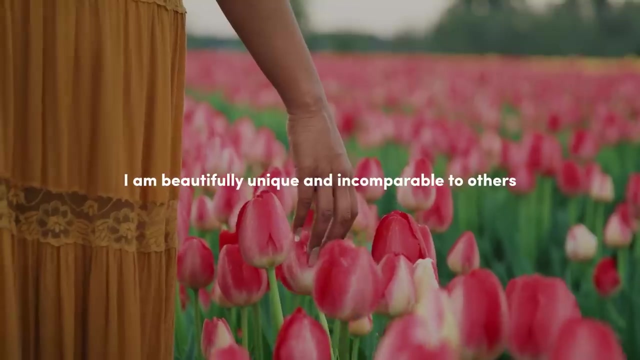 I trust myself. I believe in myself. I trust myself. I shine brightest when I am my true self. I shine brightest when I am my true self. I am beautifully unique and incomparable to others. I am beautifully unique and incomparable to others. 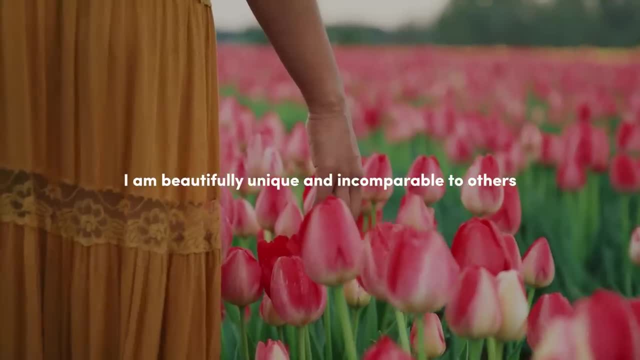 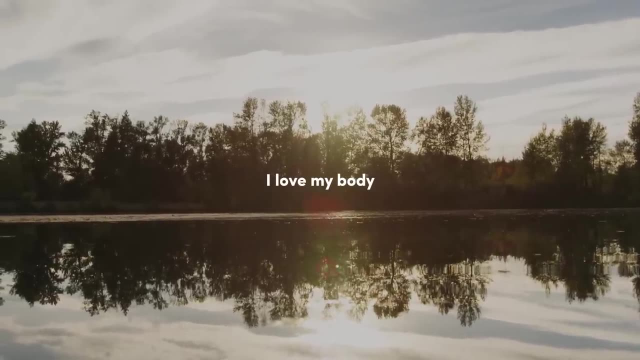 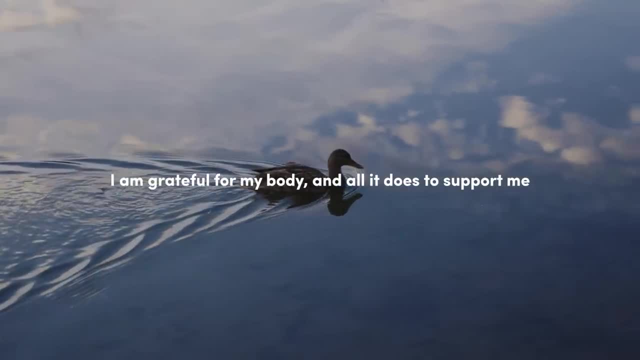 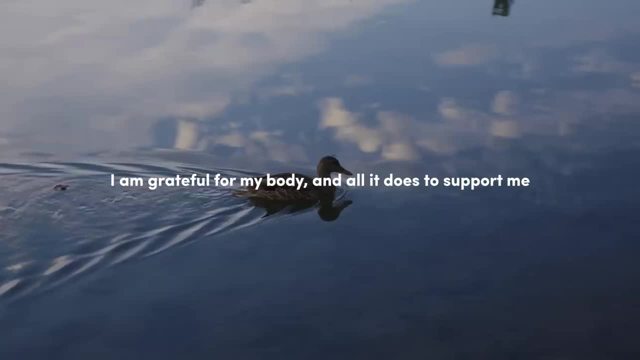 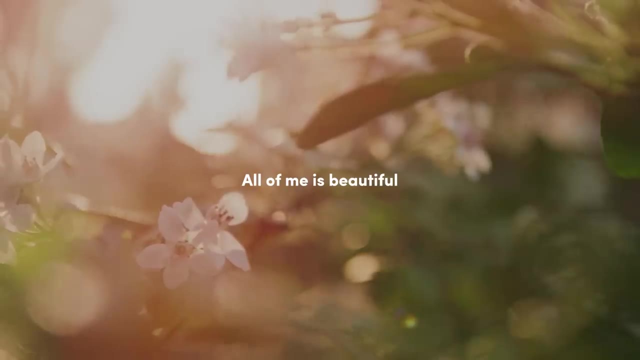 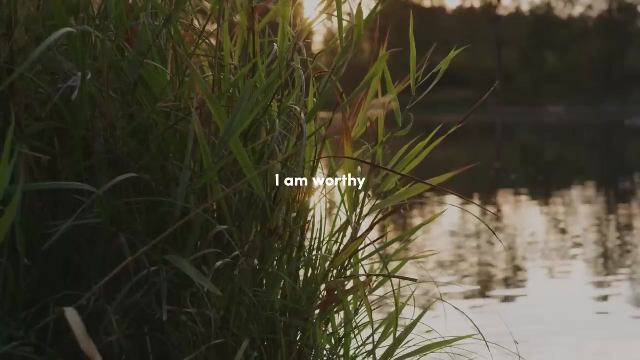 I am grateful for my body and all it does to support me. I am grateful for my body and all it does to support me. I am grateful for my body and all it does to support me. All of me is beautiful. I am worthy. 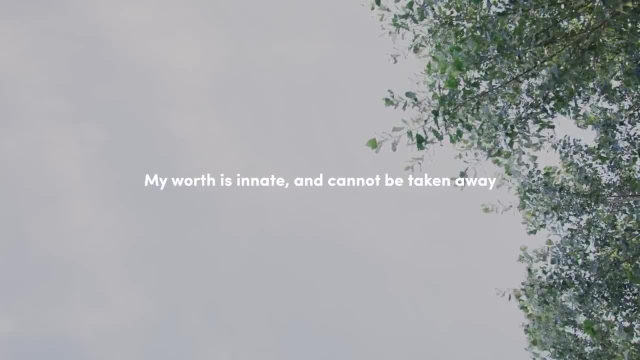 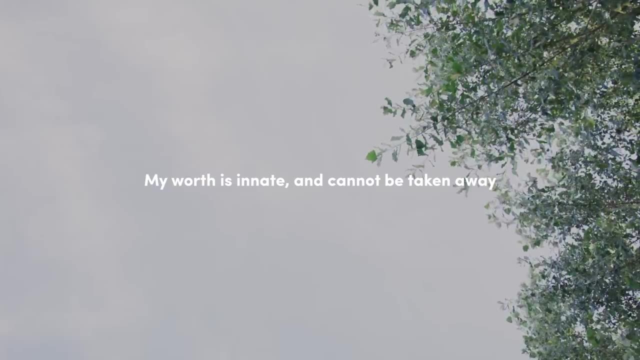 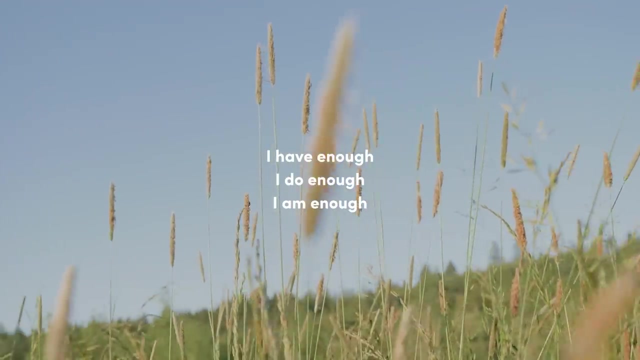 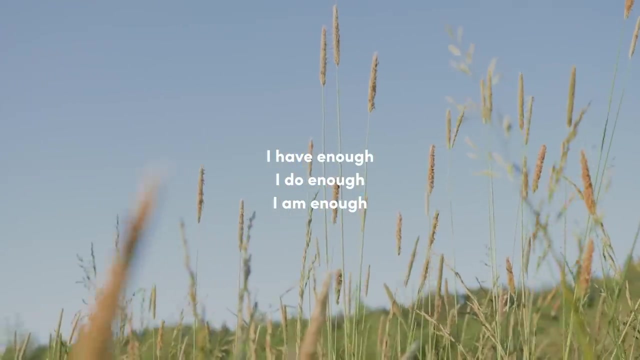 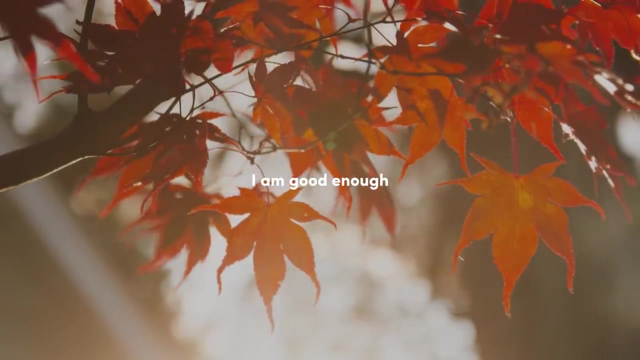 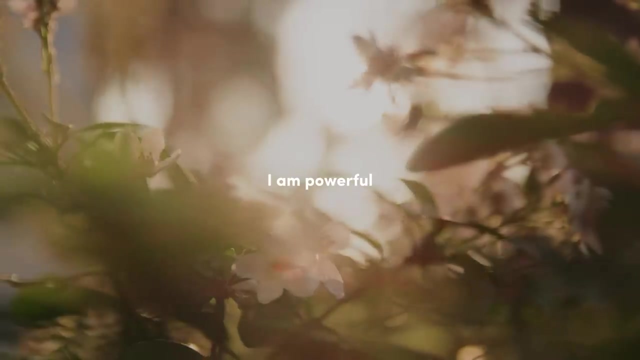 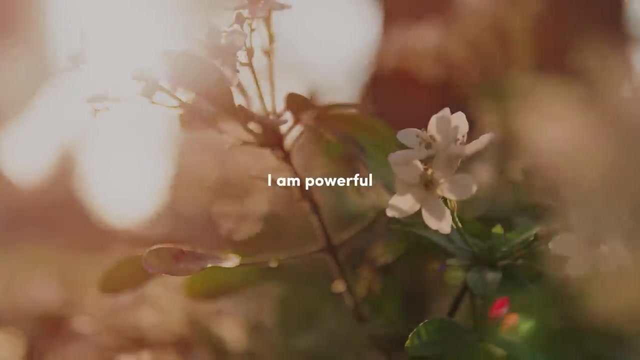 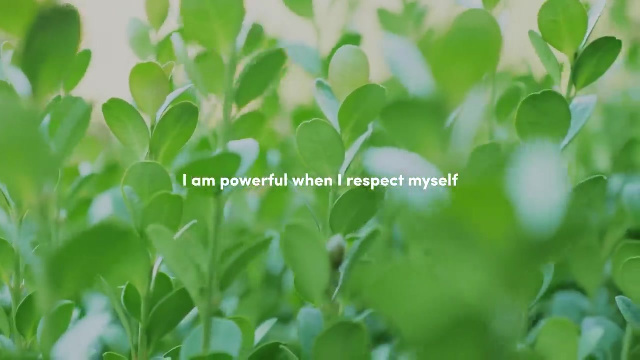 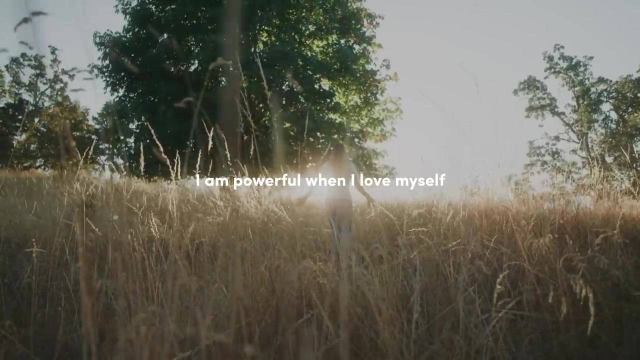 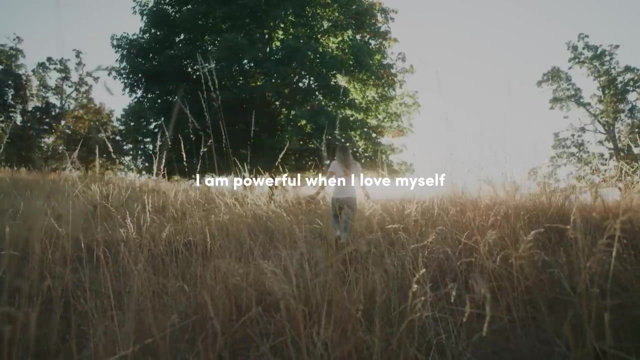 My worth is innate and cannot be taken away. I have enough, I do enough, I am enough, I am good enough. I am powerful. I am powerful when I respect myself. I am powerful when I love myself. I am a force. 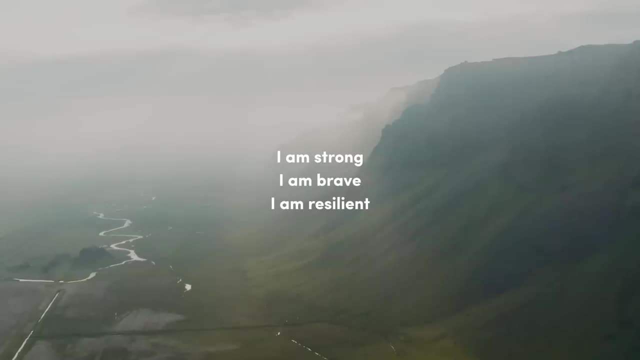 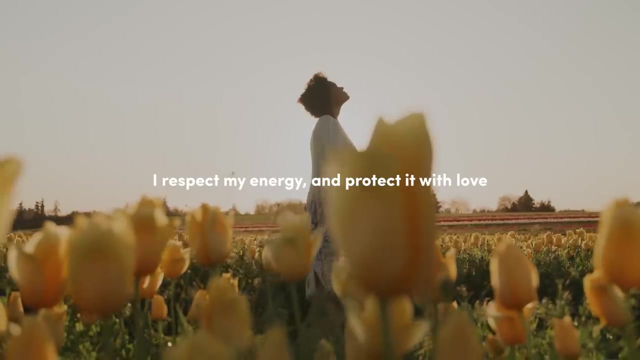 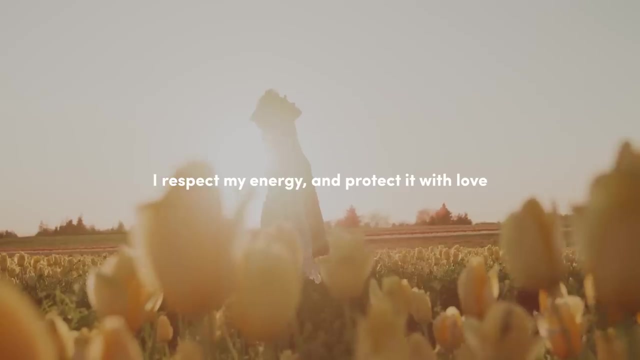 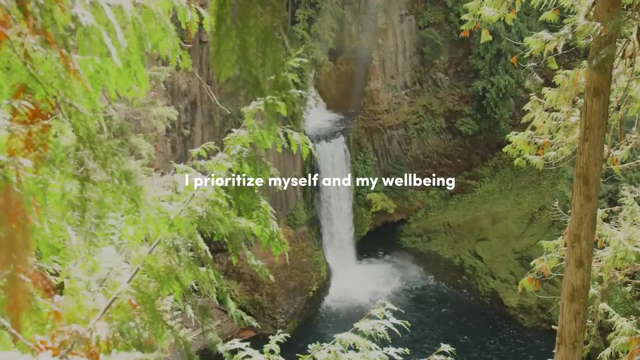 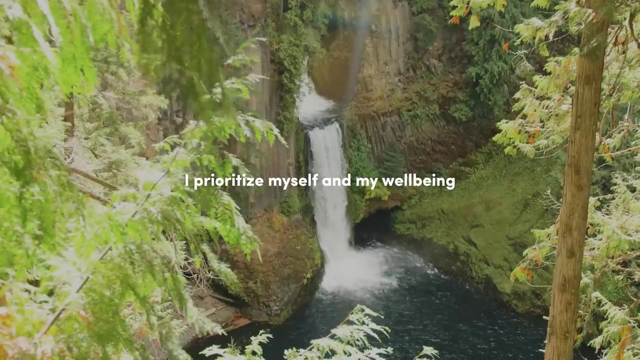 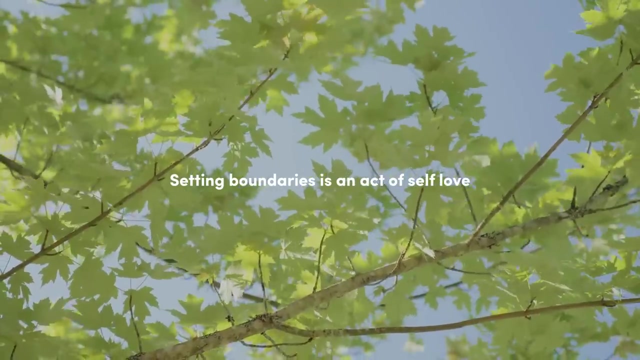 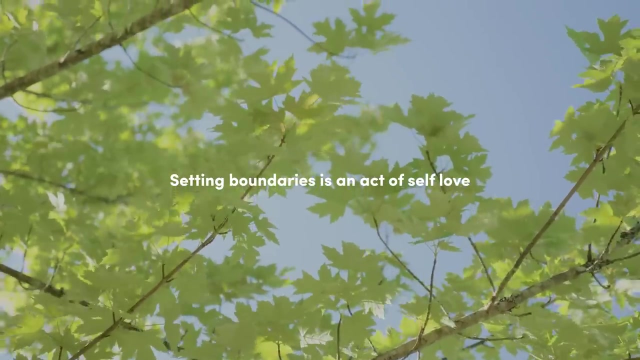 I am a force, I am strong, I am brave, I am resilient. I respect my energy and protect it with love. I prioritize myself and my well-being. Setting boundaries is an act of self-love. I love being my most authentic self. 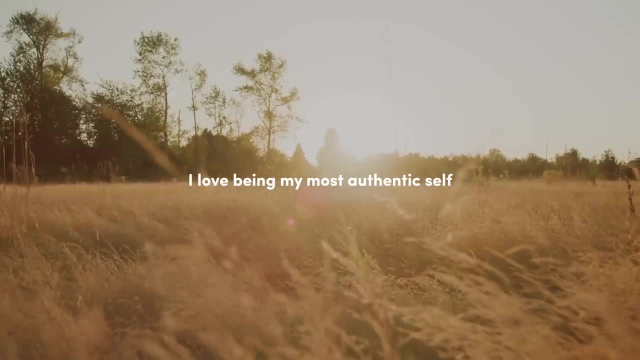 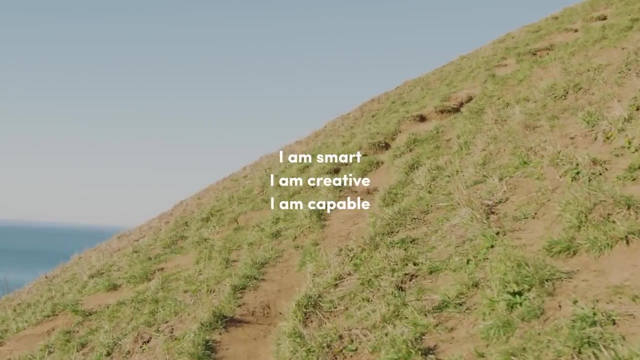 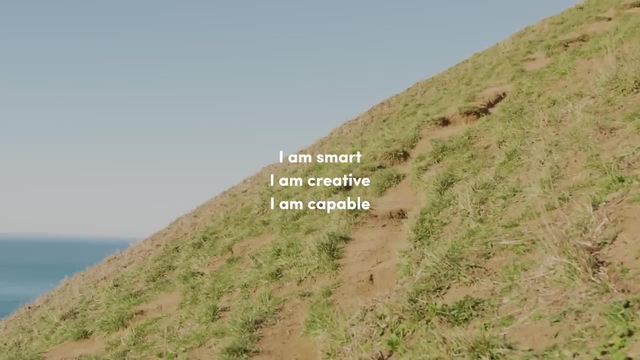 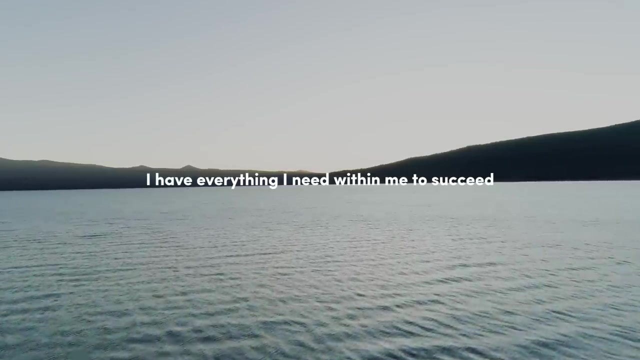 I love being my most authentic self. I am smart, I am creative, I am capable. I am smart, I am creative, I am capable. I have everything I need within me to succeed. I have everything I need within me to succeed. 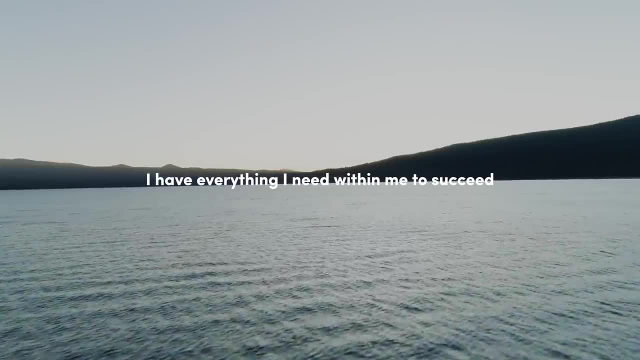 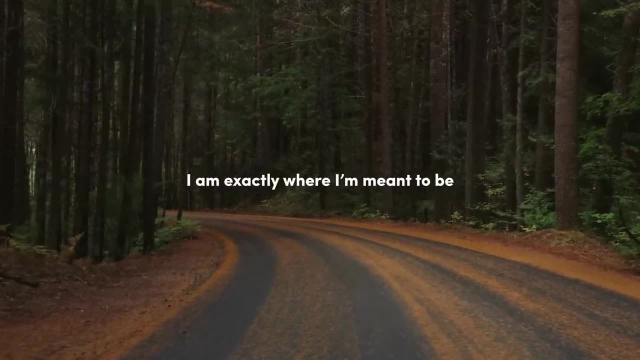 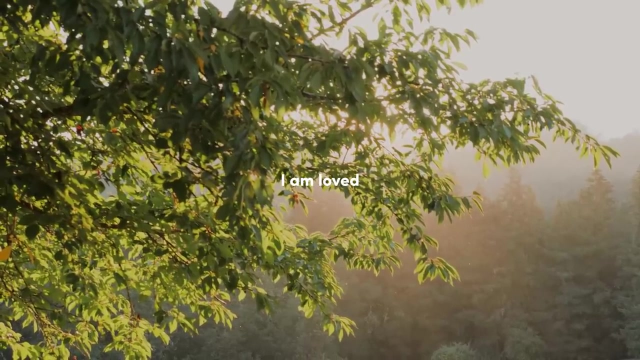 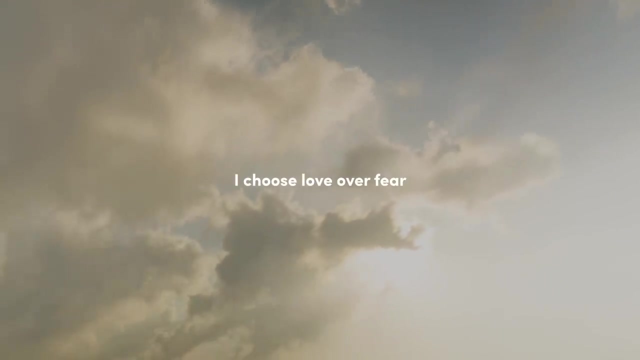 I have everything I need within me to succeed. I am exactly where I'm meant to be. I am exactly where I'm meant to be. I am loved. I am loved. I choose love over fear. I choose love over fear. I am ready to step into my true power. 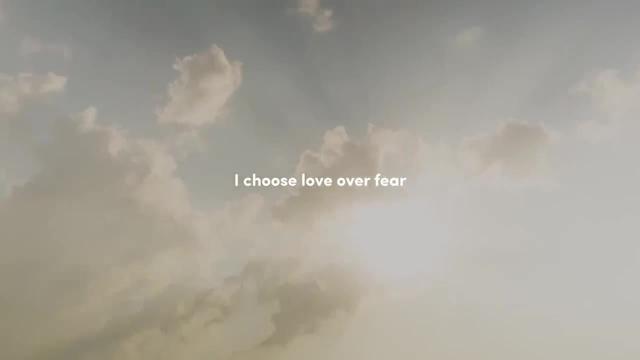 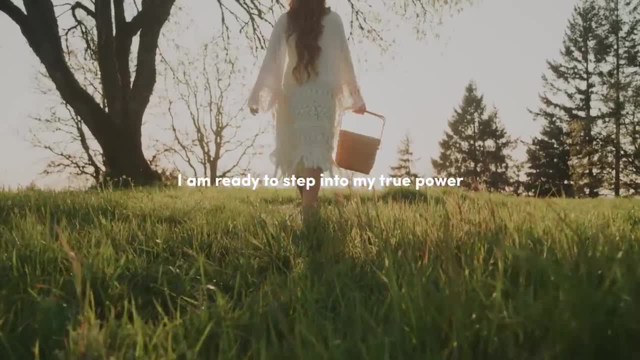 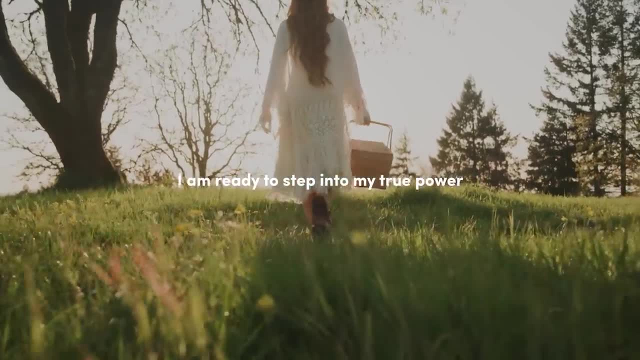 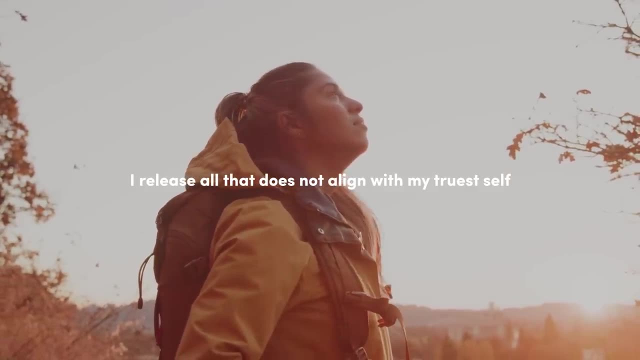 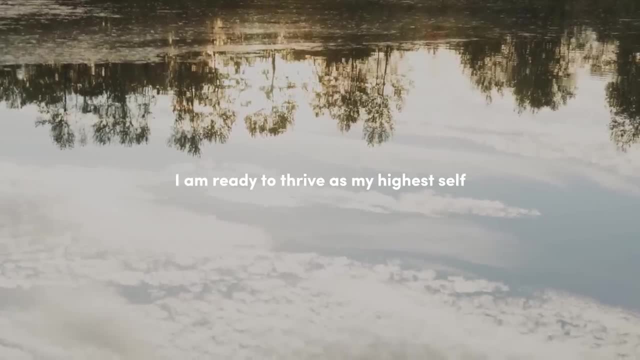 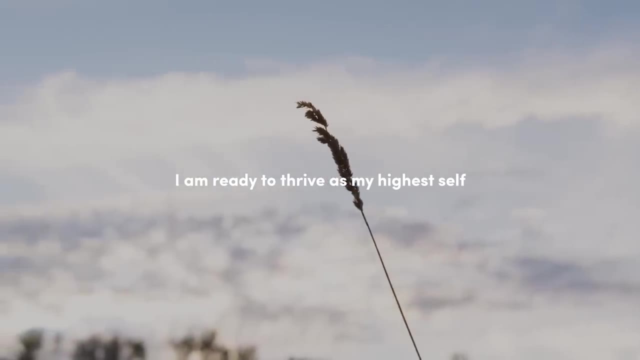 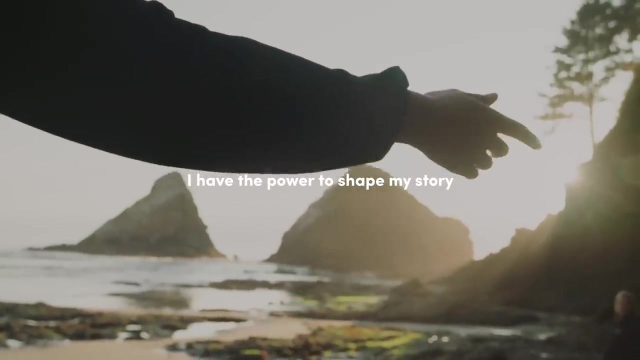 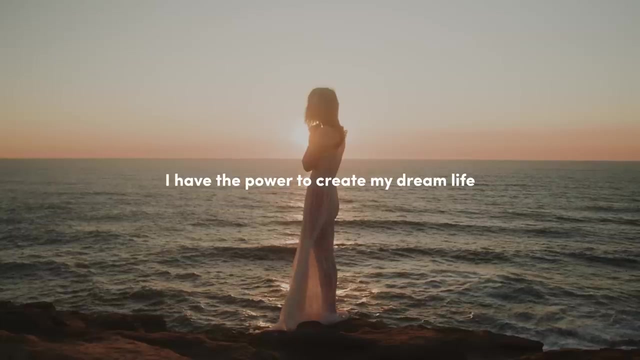 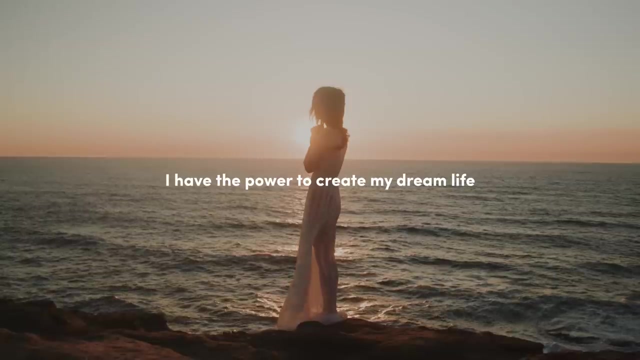 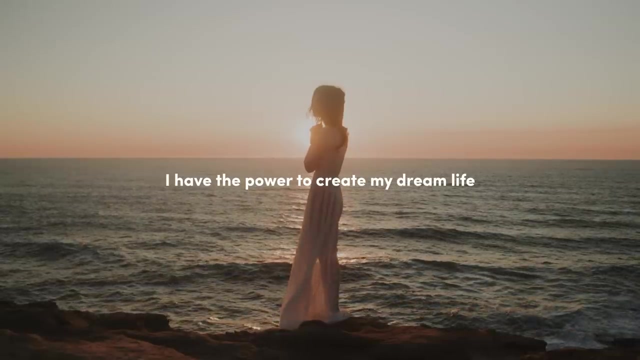 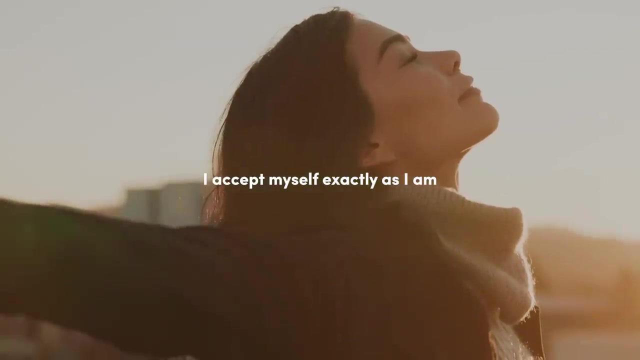 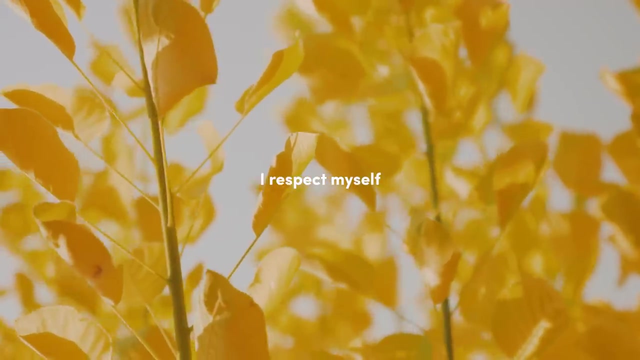 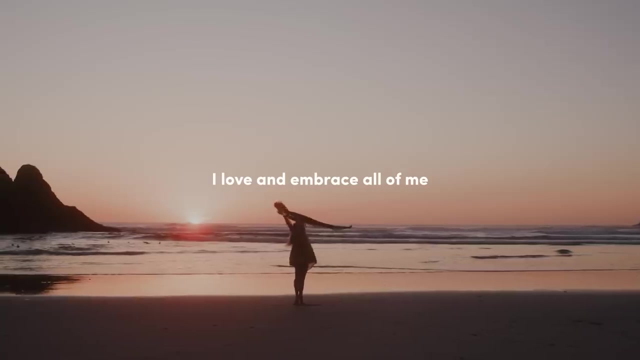 I am ready to thrive as my highest self. I have the power to shape my story. I have the power to create my dream life. I accept myself exactly as I am. I respect myself. I love and embrace all of me. I love and embrace all of me. 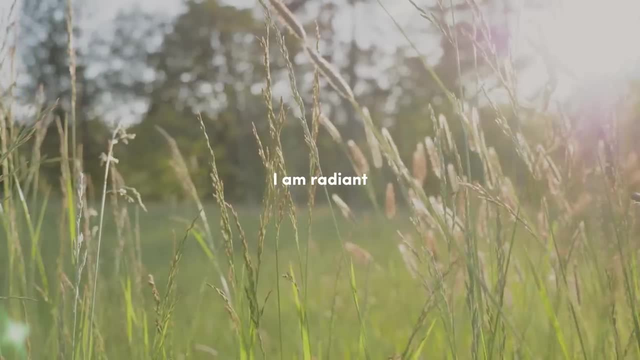 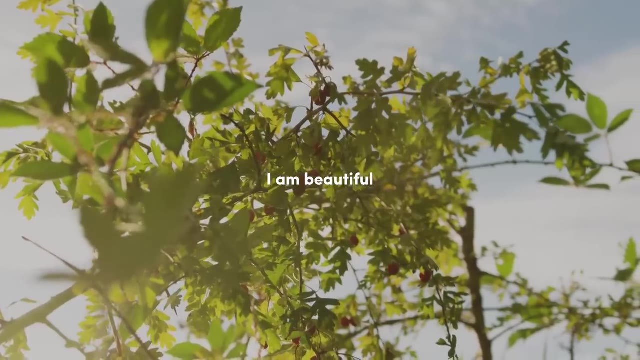 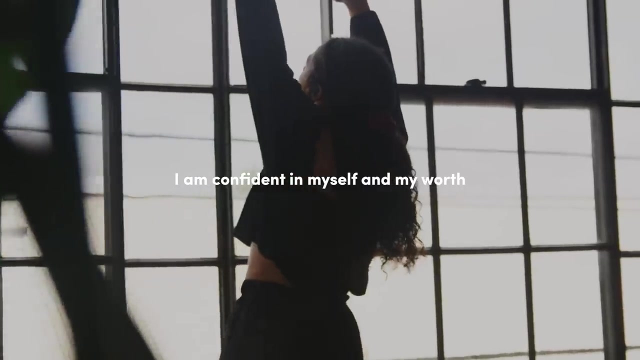 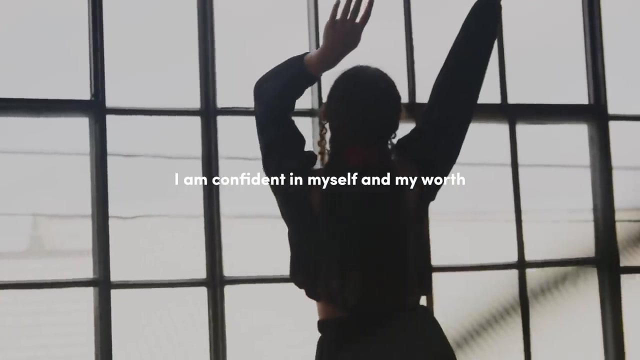 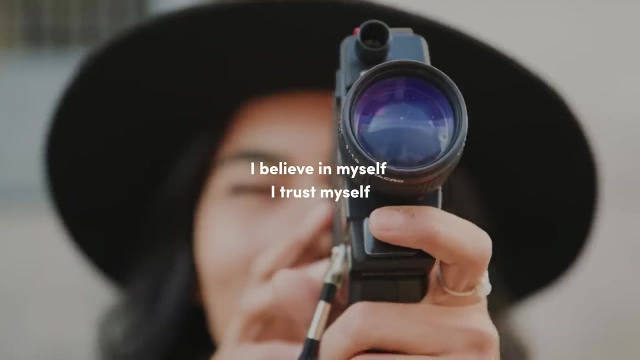 I am radiant. I am radiant. I am beautiful. I am beautiful. I am confident in myself and my worth. I am confident in myself and my worth. I believe in myself, I trust myself. I believe in myself, I trust myself. 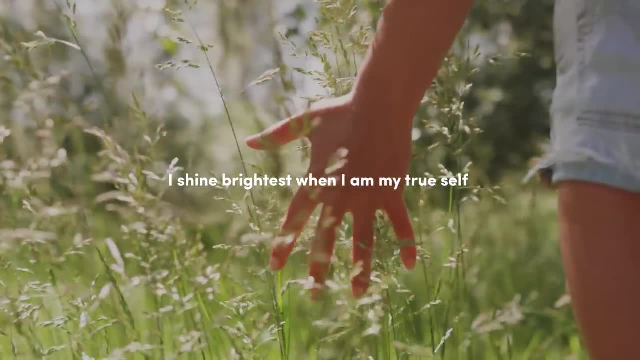 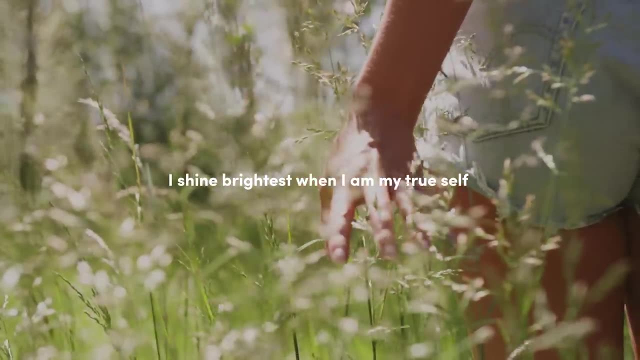 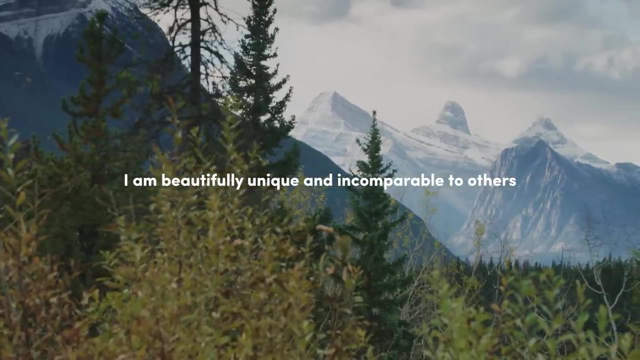 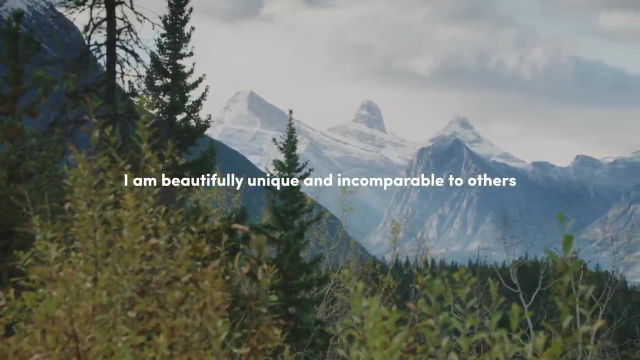 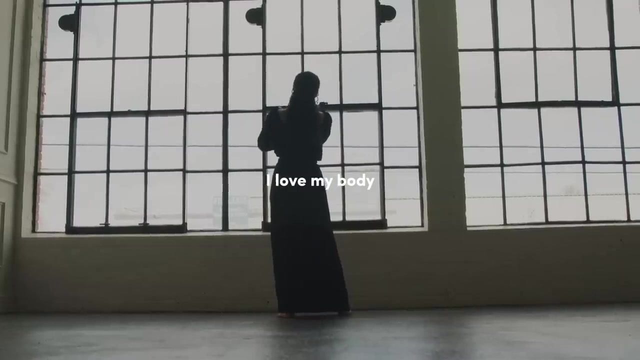 I shine brightest when I am my true self. I shine brightest when I am my true self. I am beautifully unique and incomparable to others. I am beautifully unique and incomparable to others. I love my body. I love my body. I am grateful for my body and all it does to support me. 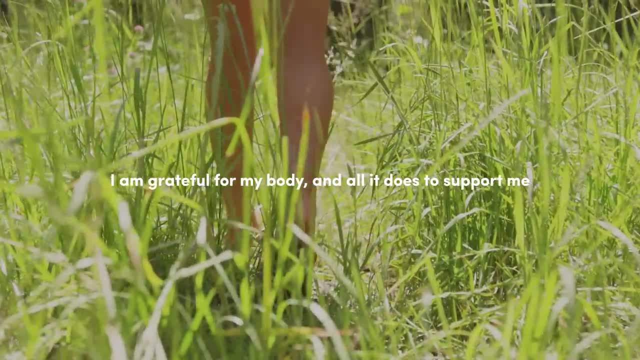 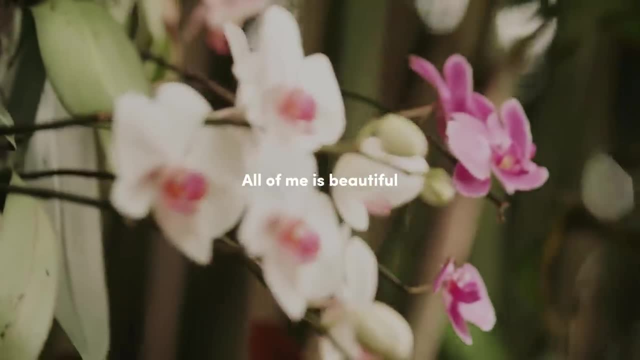 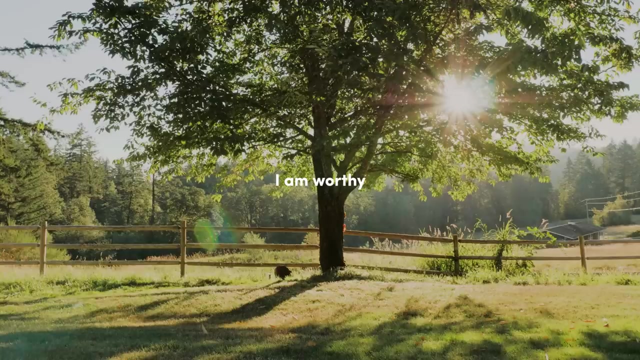 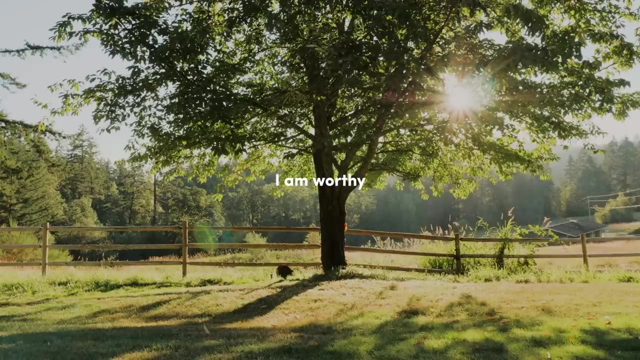 I am grateful for my body and all it does to support me. All of me is beautiful. All of me is beautiful. I am worthy. I am worthy, All of me is beautiful. My worth is innate and cannot be taken away. 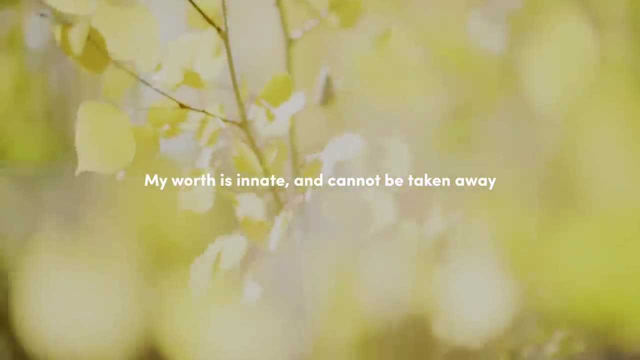 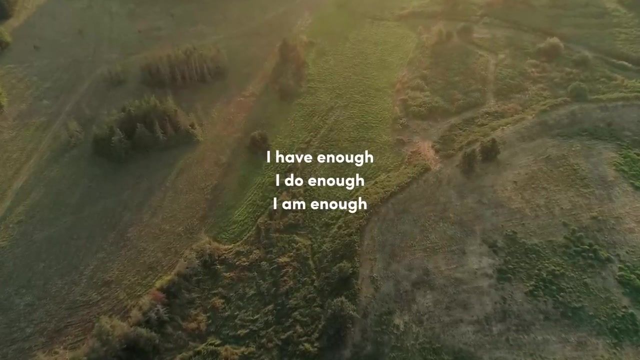 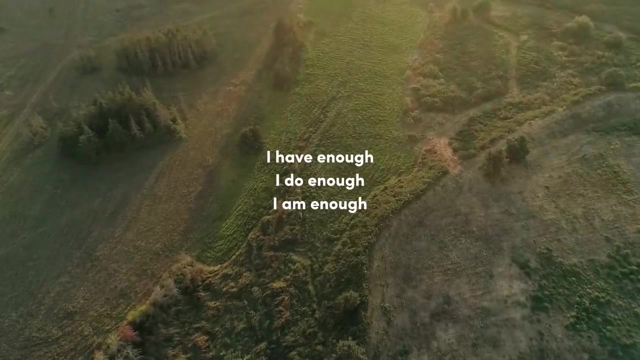 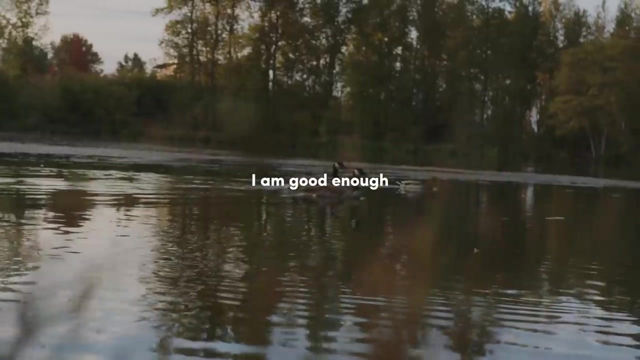 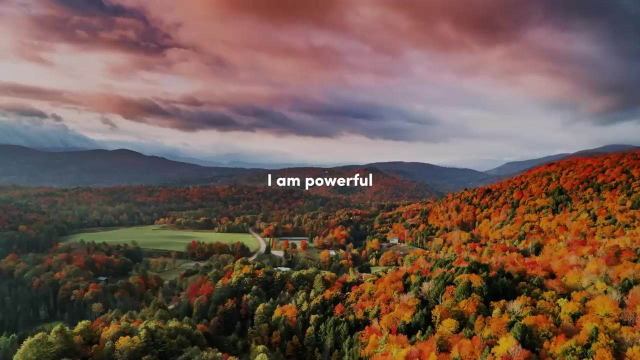 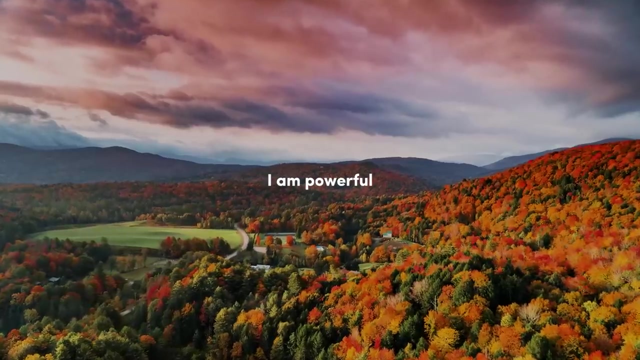 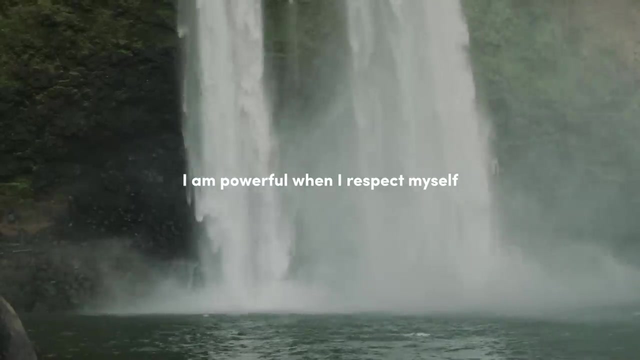 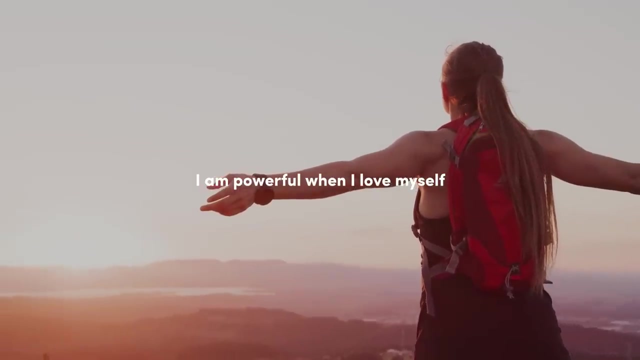 My worth is innate and cannot be taken away. Sevenooo Eicshāsi, I have enough, I do enough, I am enough, I am good enough, I am powerful. I am powerful when I respect myself. I am powerful when I love myself. 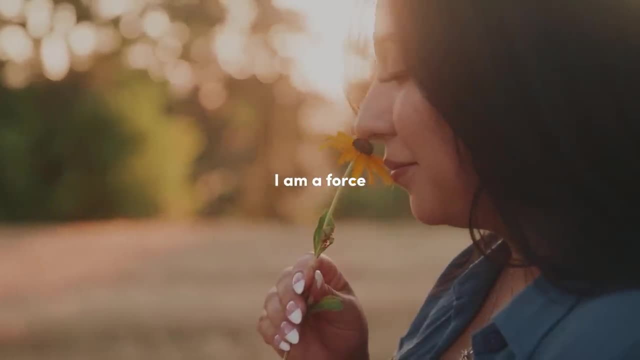 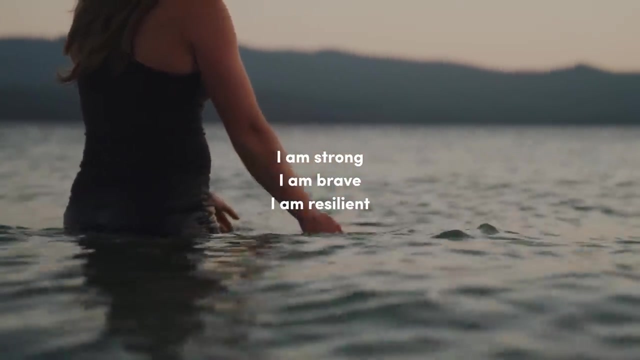 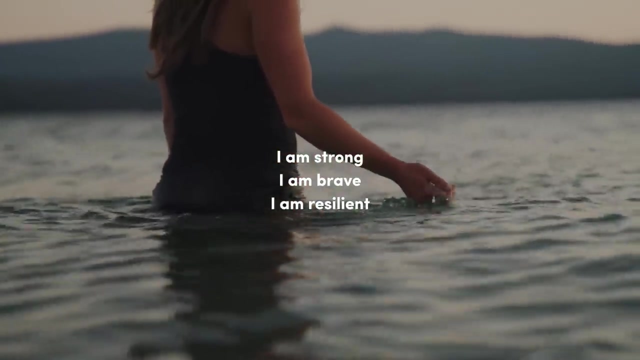 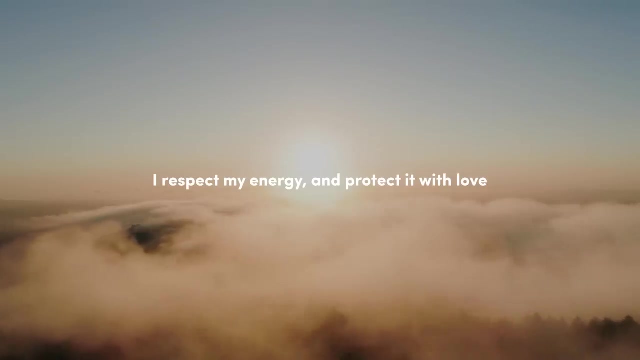 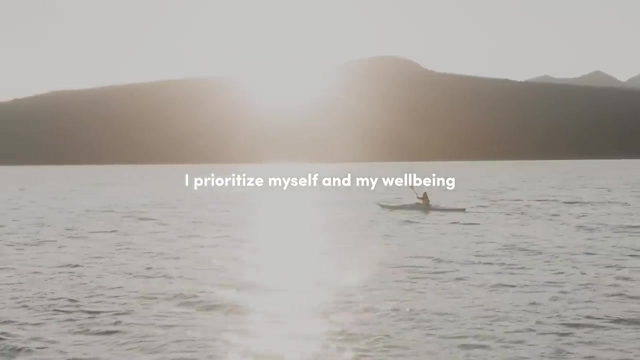 I am a force, I am strong, I am brave. resilient. I am strong, I am brave, I am resilient. I respect my energy and protect it with love. I respect my energy and protect it with love. I prioritize myself and my well-being. I prioritize myself and my well-being. 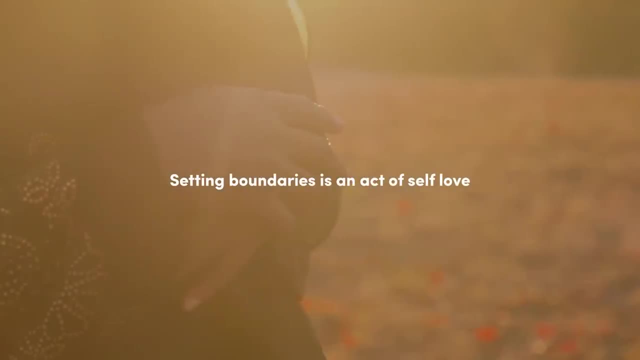 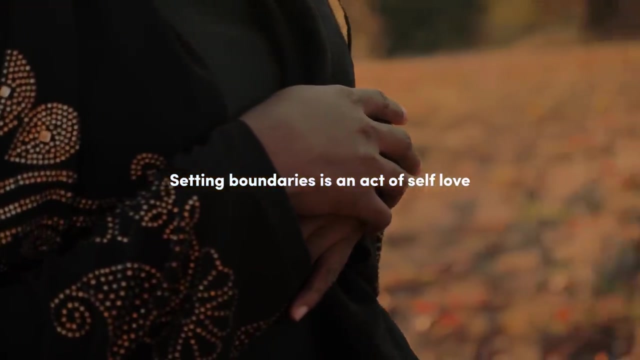 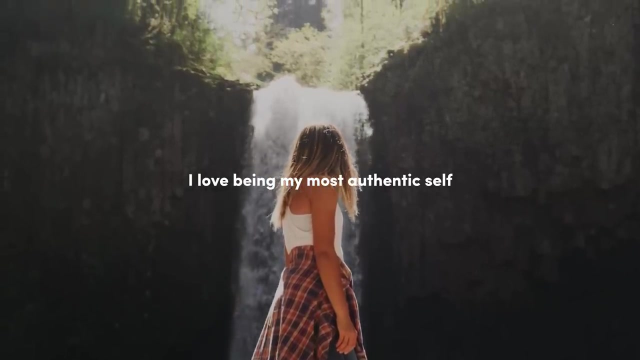 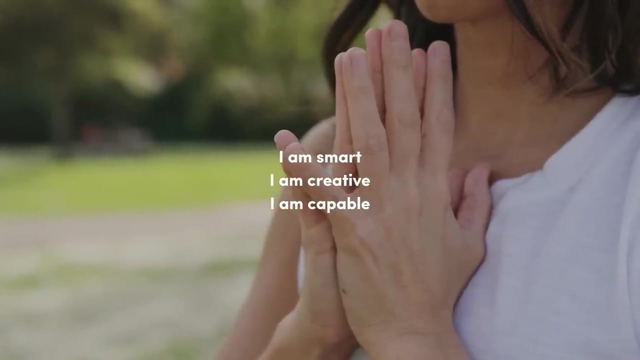 Setting boundaries is an act of self-love. Setting boundaries is an act of self-love. I love being my most authentic self. I love being my most authentic self. I am smart, I am creative, I am capable. I am smart, I am creative, I am capable. 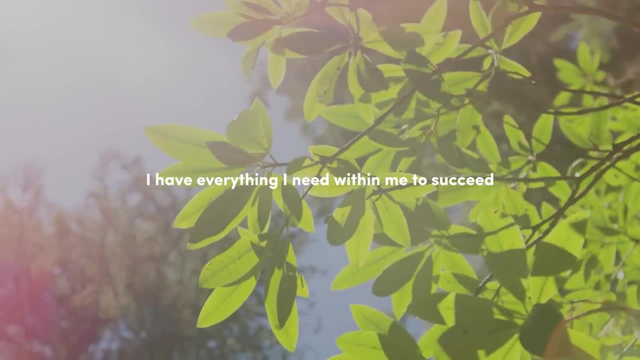 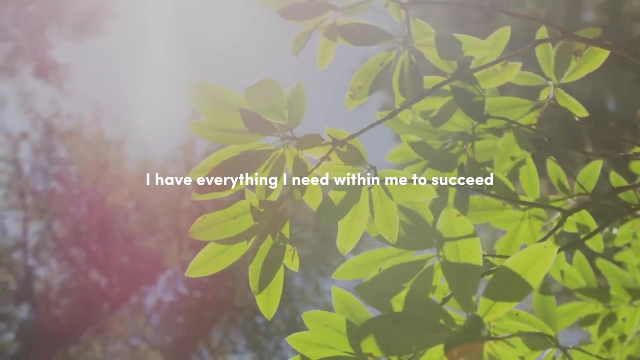 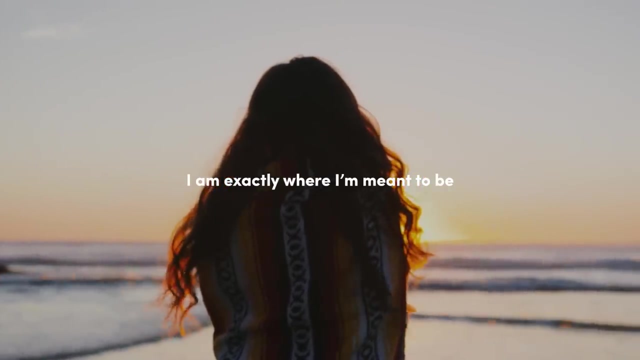